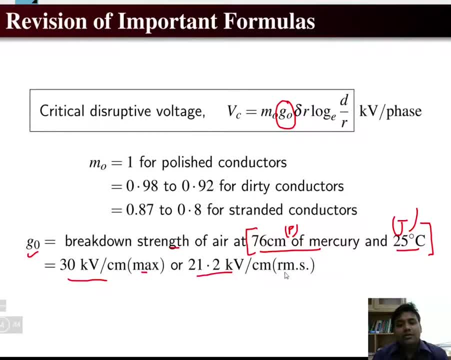 to the maximum value, or 21.2 kilo volt per centimeter. that is the rms value. Since all the calculations are ac, so we will be calculating the values in terms of rms. So 21.2 kilo volt per centimeter will be used for the value of g0.. The value of delta, that is the air density factor. 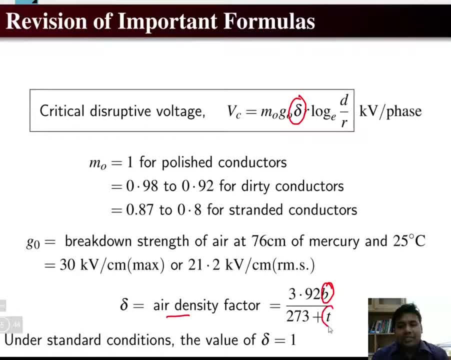 depends upon the pressure v and the temperature t. So the formula is 3.92 v, 273.. plus temperature, whereas for the standard condition the value of delta is one other conditions. the value of delta will be given. The r is basically the radius of the conductor. 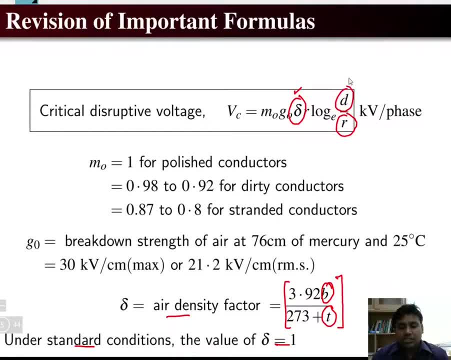 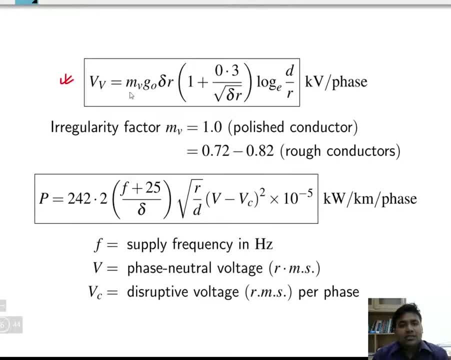 and d is the distance of separation between the conductors. The next formula that we will use is the visual critical voltage. This depends upon one more irregularity factor, mv, whose value is 1 for polished conductor and 0.7 to 0.8 to for rough conductors. 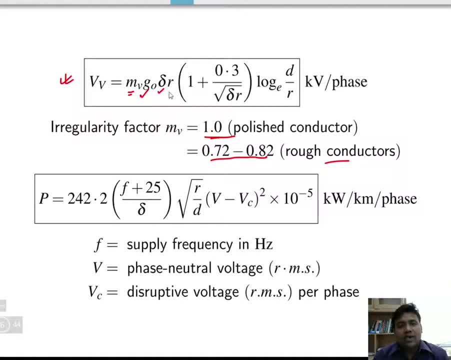 g0. we have already calculated delta. we have calculated r is the radius of the conductor, and the rest of the formulas is this: All the formulas will be calculated on the basis of per phase and the unit is in kilo volt. Next formula is the power loss formula. So this is: 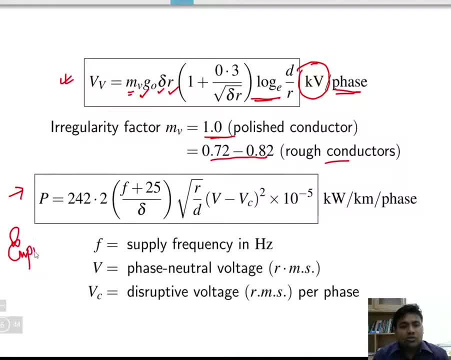 the empirical formula that is used to solve the corona loss. empirical formula. So it is used to solve the corona loss. So it is 242.2 kilo volt per centimeter. So this is the empirical formula. Next formula is the frequency plus 25 divided by delta under root r, by d. v is the phase to. 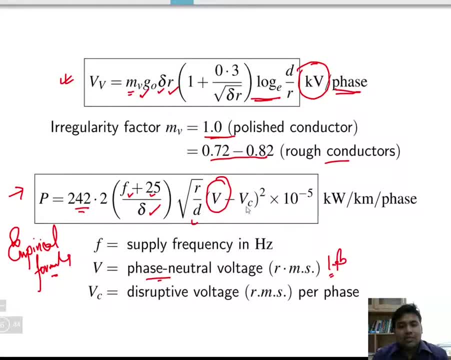 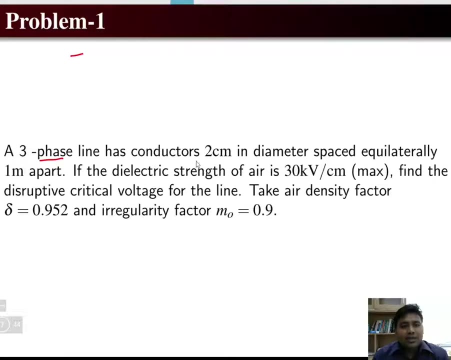 neutral voltage because it is in single phase and this is the rms. vc is the critical voltage, that is also in rms per phase and f is the supply frequency. The unit is in kilo watt per kilometer per phase. Problem number one: if you have a three phase line conductors having two centimeter in. 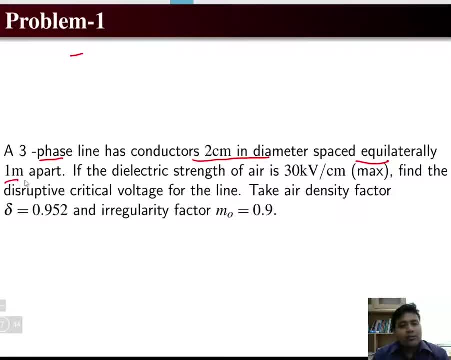 diameter, spaced equilaterally. If the dielectric strength of air is 30 kilo volt per centimeter maximum, find the disruptive critical voltage of the line. Take air density factor delta to be 0.952 and irregularity factor 0.9.. Now, since it is a three phase line, we have to convert all the quantities into single phase. 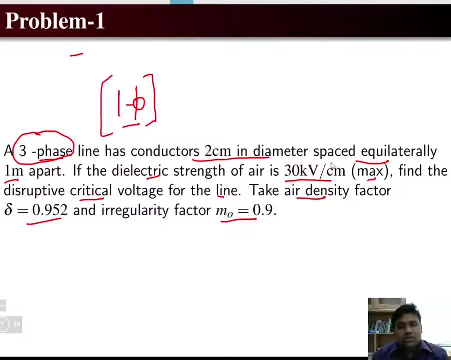 and then solve the problem. So these 30 kilo volt per centimeter maximum we have to obtain 21.2 kilo volt per centimeter. So this is the critical voltage of the line. So this is the critical voltage, rms, as the rms quantity and all the voltages, we have to convert it into single phase, So conductor. 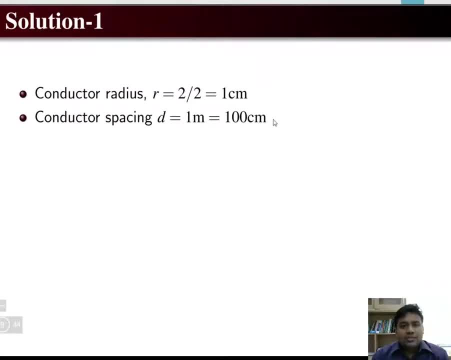 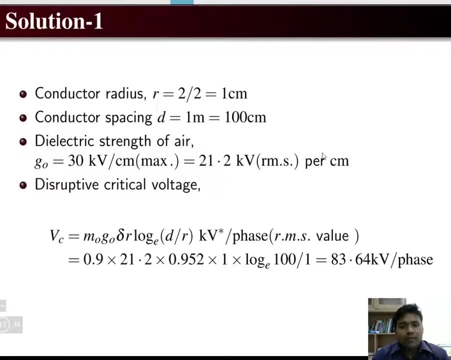 radius is one centimeter, Spacing is 100 centimeter. Dielectric strength of air will take 21.2 kilo volt per centimeter. Then we can use the formula: vc is equal to m naught, g naught, delta, r, log e, d by r, So the unit is in kilo volt, because the value of g naught is in kilo volt. So this is: 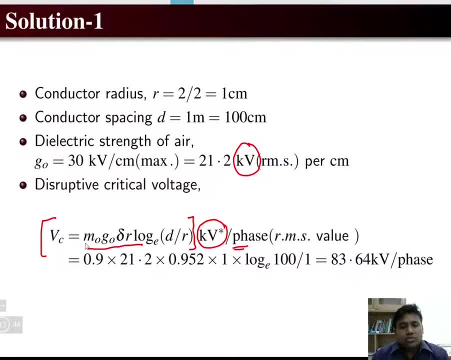 in kilo volt, And here we have per phase calculations. So, substituting all those values, we will get a answer: 83.64 kilo volt per phase. Now, since the answer has to be represent in the line values for three phase quantity, we have to multiply this with root 3 into 83.64.. So we are. 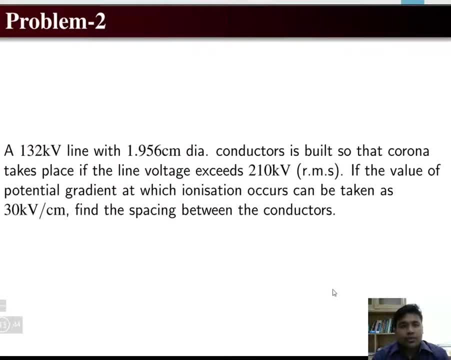 getting 144.8 kilo volt. Problem number two: if you have a 132 kV line, the diameter is 1.2, 9.56 is built so that corona takes place if the line voltage exceeds 210 kilo volt rms. So once the 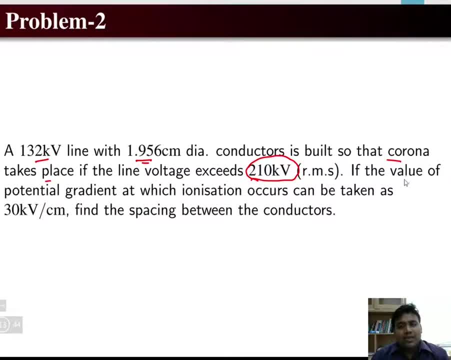 voltage exceeds 210 kilo volt, the corona will take place If the value of the potential gradient at which ionization occur can taken as 30 kilo volt per centimeter. So this is the value of g naught maximum. So you have to convert into rms, Find the spacing between the conductor d. So what is the? 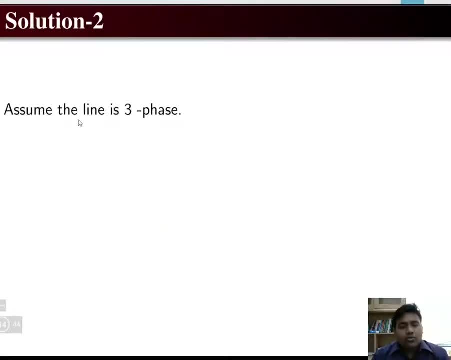 spacing between the conductor. So you have to convert into rms. So you have to convert into rms, So you have to assume that the line is in three phase. So the radius of the conductor first we have to obtain. Then the dielectric strength of air g naught is 21.2 kilo volt rms per centimeter. 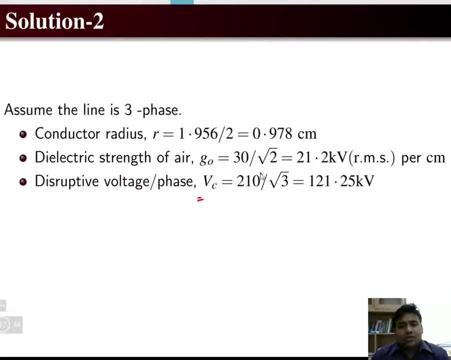 Then the disruptive critical voltage, since once the 210 kV it cross. but that is a three phase line, so you have to obtain the per phase basis, So it will be 121.25 kilo volt per phase. Then no conditions has been given about the conductor, So you have to assume that it is a 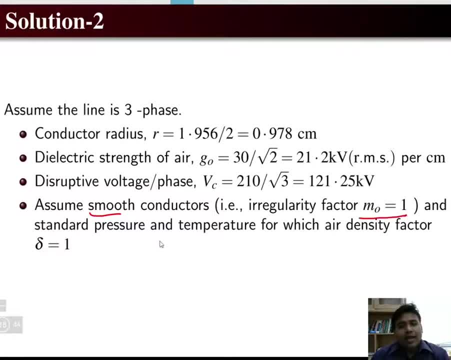 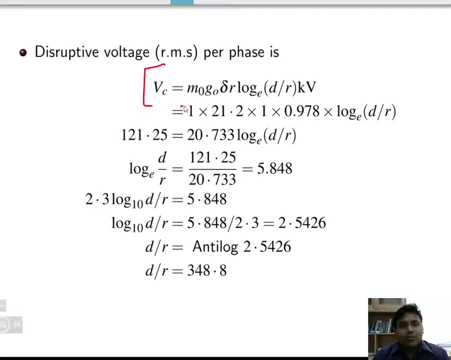 smooth conductor, So irregularity factor will be 1 and the conditions are standard pressure and temperature conditions, So air density factor will be 1.. Then, if d centimeter is there the spacing between the conductor, then using the formula for critical disruptive voltage as this, substituting: 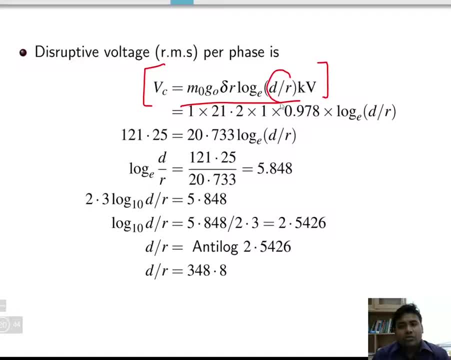 all the values except d by rm. So this is the formula for critical disruptive voltage. So this is d by rm. So we will leave d by rm as such. so we can obtain d by rm as 348.8, because we are already given all these quantities. So taking the anti-lock value, you can get 348.8.. So, multiplying with the, 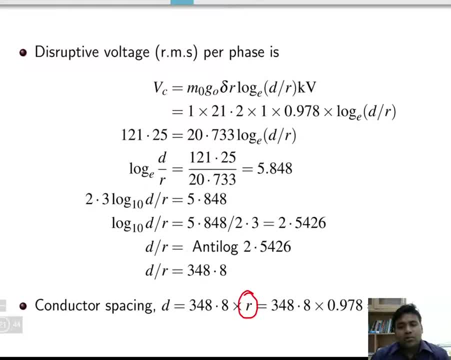 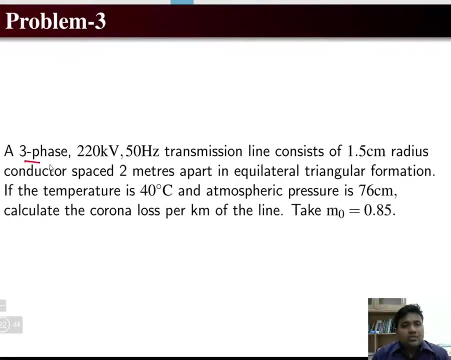 radius of the conductor which is given to you, you get 341 centimeter as the conductor spacing. Problem number three: a three phase 220 kV, 50 hertz transmission line consists of 1.5 centimeter radius conductor space 2 meter apart. 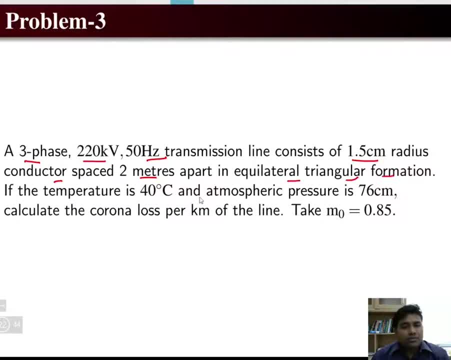 in equilateral triangle formation: temperature: 40 degree centigrade pressure: atmospheric pressure: 76 centimeter. You have to find the corona loss per kilometer of the line. take m naught to be 0.85.. So here the system is in three phase. So this corona loss calculation has to be in three phase. 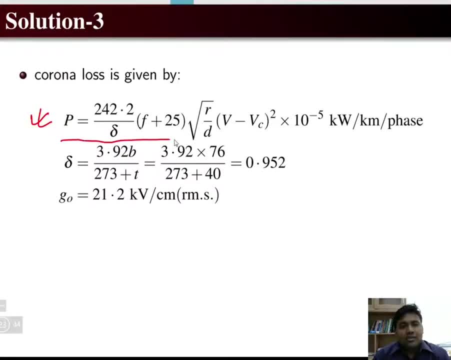 So the corona loss formula is this which we have seen, and here we require the value of delta. So delta depends upon the pressure and temperature. So substituting the pressure and temperature we get the value of delta as 0.952 and g naught we know that is 21.2 kilovolt per centimeter. 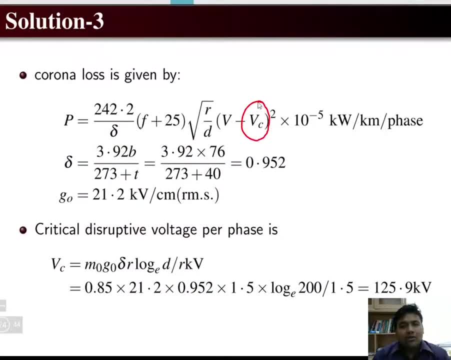 So critical disruptive voltage we will be requiring to find the values of corona loss, So critical disruptive voltage formula we have seen. So putting that formula, We will get a value 125.9 kV and then we can substitute here Vc. 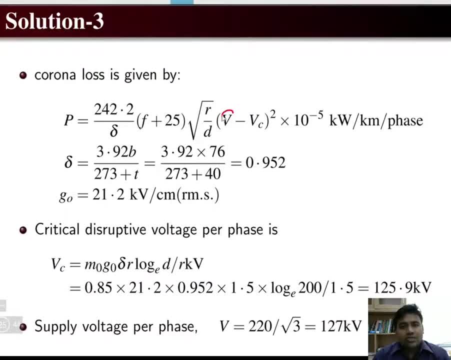 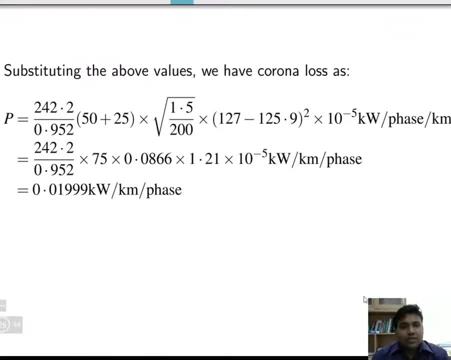 So supply voltage per phase, because here the voltage has to be in per phase and the given voltage is 220.. So divided with root 3 you get 127 kV. After that we know all the data so that you substitute in the power loss. 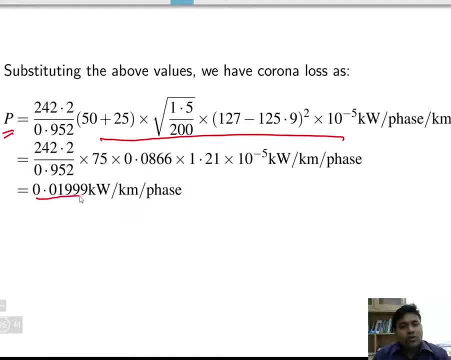 formula and the final answer will be 0.0199 kilovolt per kilometer per phase. However, since it is a three phase system, we have to convert the single phase into three phase. So that can be done by multiplying it with three times. Three times the single phase, power loss will get a total of 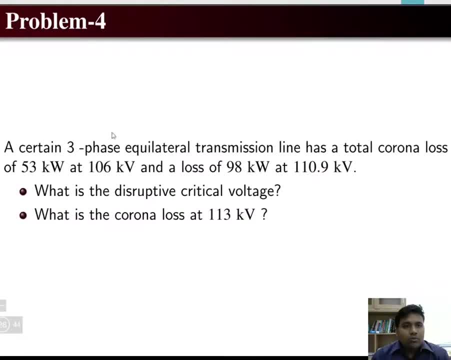 0.06 kW. Problem number four is certain three phase equilateral transmission line has a total corona loss. So total corona loss is given 53 kW at 106 kV and loss of 98 kW at 110.9 kW. So total corona loss is given 53 kW at 106 kV and loss of 98 kW at 110.9 kV. So total corona loss is given 53 kW at 106 kV and loss of 98 kW at 110.9 kV. 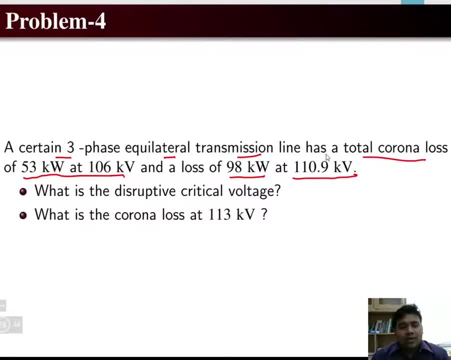 So total corona loss is given 53 kW at 110.9 kV and loss of 98 kV at 110.9 kV. No information is given about the other factors of the conductor, So that has to be taken as constant. 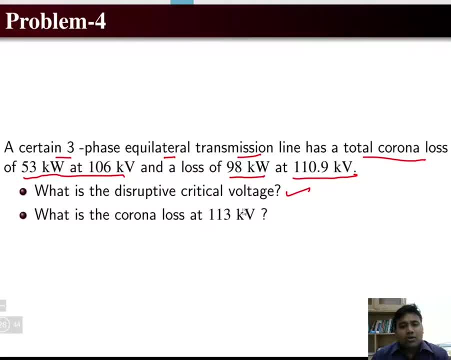 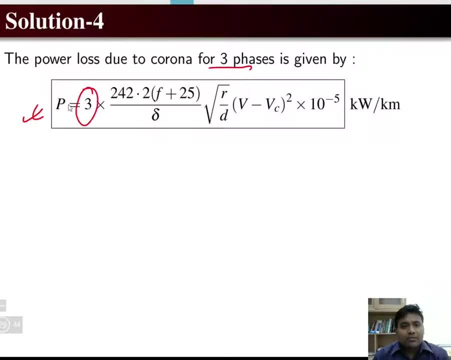 What is the disruptive critical voltage and what is the corona loss at 113 kV? So the formula for corona loss for a three phase we have multiplied with three with the single phase formula. So here we can see that except V and Vc, that is, a supply voltage and disruptive critical voltage, other factors are same for the two cases. 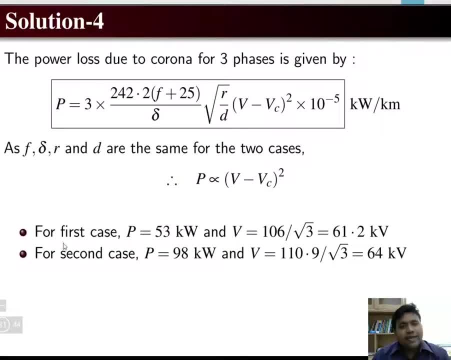 So we have can make the two case where the power loss is 53 kW and 98 kW. So here the voltage has to be converted into: per phase, 106 divided by root 3 and 110.9 divided by root 3.. So these are corresponding to single phase voltage. 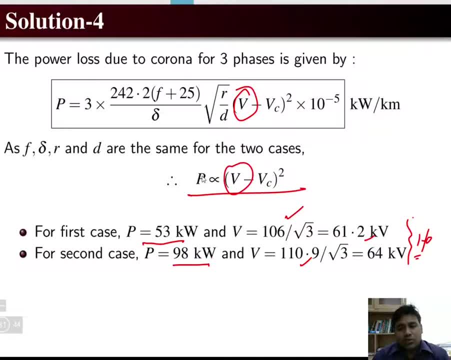 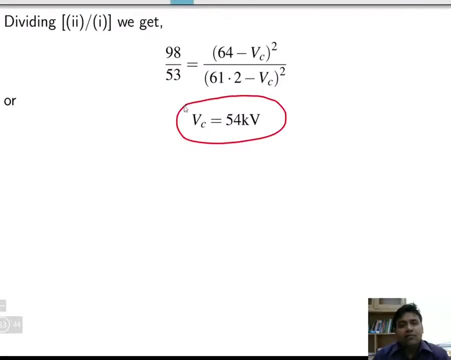 So that we can substitute here as the formula for voltage and we can form two case, case number 1 and case number 2.. So here we are getting Two cases of power. if we divide the two case then we can easily obtain the value of critical voltage Vc as 54 kV. 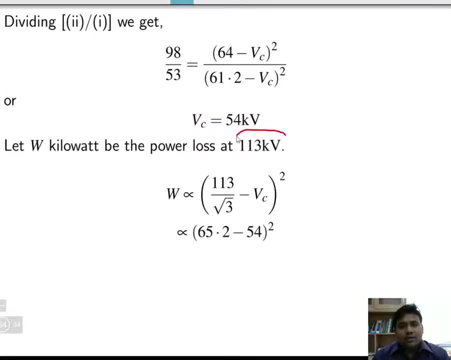 The third case was given to be 113 kV. What is the power loss? So, similarly, here we can put 113 by root, 3 minus Vc, So dividing the equation 3 and 1.. So this is the third equation with the first equation, if you divide, and the power loss is coming. 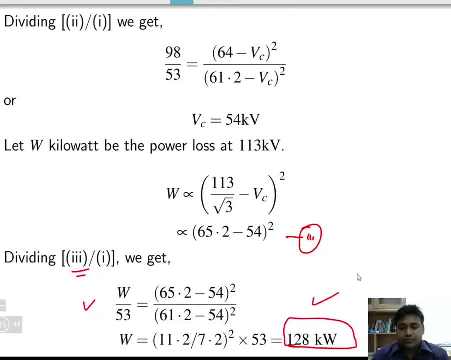 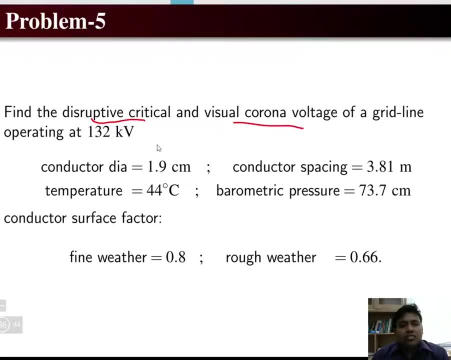 To be 128 kW. Problem number fifth and the last problem is find the disruptive, critical and visual corona voltage of the grid line operating at 132 kV. So this is basically a three phase transmission line where the voltage operating is 132 kV or the specification of the conductor, diameter, temperature, spacing and pressure is given. 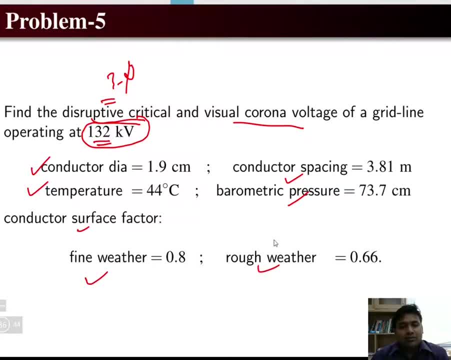 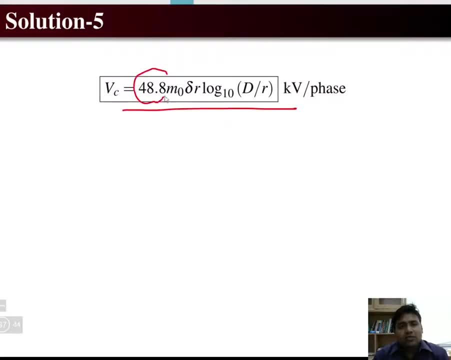 Conductor surface for the fine weather and rough weather conditions is given, We have to Find the disruptive critical voltage, whose formula is this: We have taken all the constant 48.8, considering the value of G, not as 21.2.. So if we substitute the value of M, not to be 0.8, and delta, we obtain, for a pressure and temperature conditions, 0.91.. 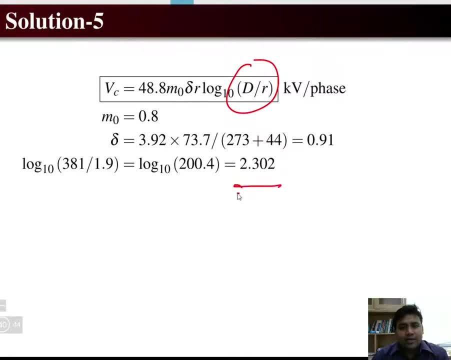 So we get log D by R. We can easily obtain 2.302.. So the visual critical disruptive voltage will be 153 kV. So we can easily obtain 2.302.. So the visual critical disruptive voltage will be 153 kV. 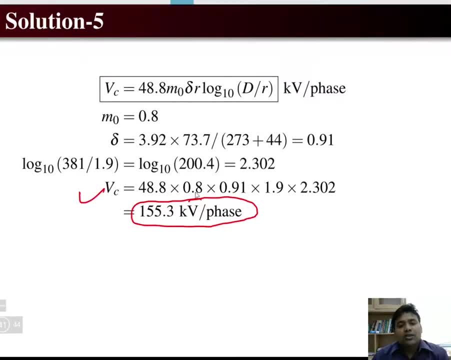 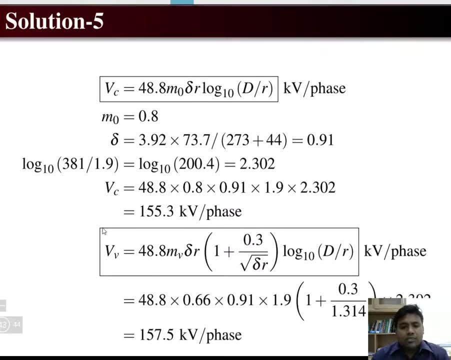 So we can easily obtain 2.302.. So the visual critical disruptive voltage will get 153 kV, so we get 350.. And the visual critical voltage we can again obtain by substituting all the values will get 157.5 kV. 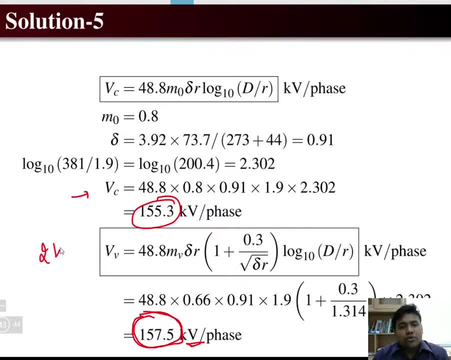 So here we can see that the critical voltage is 155.3.. And the visual critical voltage is 157.5.. So there is a difference of 2 kV insufficient. So legislature is no better configuration. So therefore we have to consider two values here. 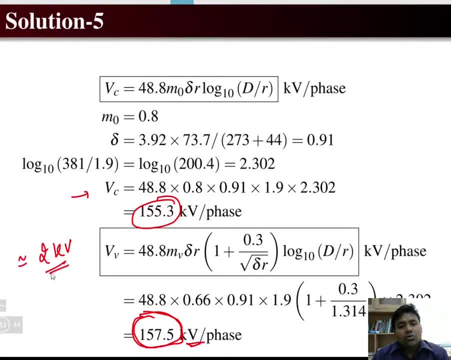 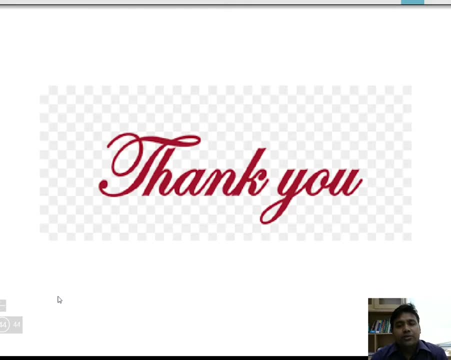 on an approx. 2 kilovolt difference is there to visualize the corona. So we required a voltage of 2000 volt to easily see the corona through the naked eye. So that's complete the tutorial on corona discharge in transmission line. Thank you.